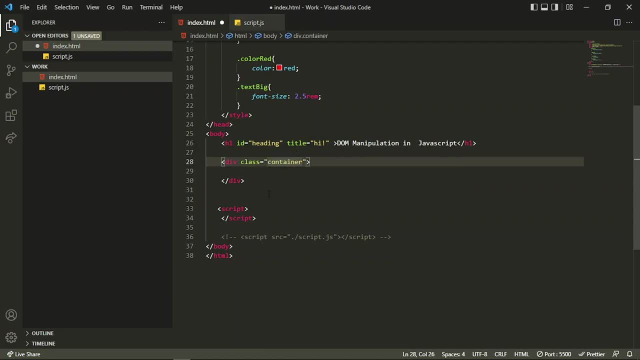 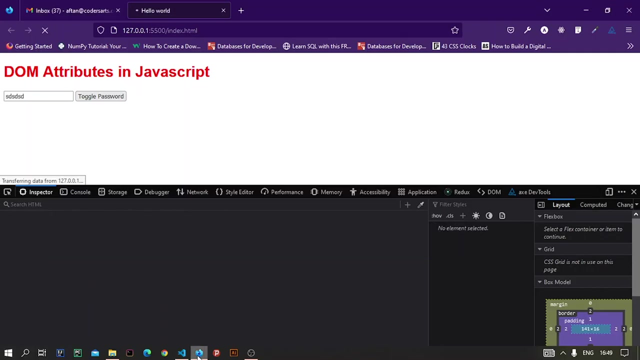 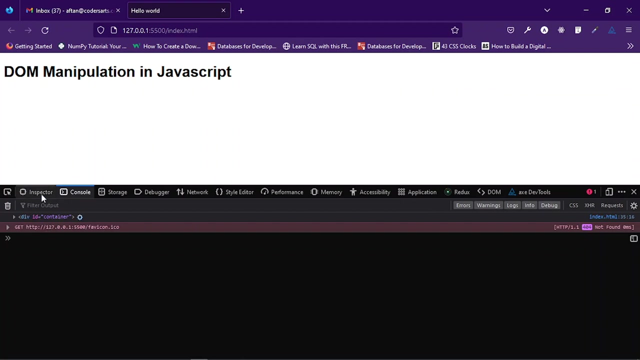 add some ID here. Let's say container. Now if I store it ID, Let's store it in a container by using documentgetElementById, and if I specify the container here, So this item will be grabbed out, right, Let's see that. So if I see the console now, you can see we have this container element and we also have 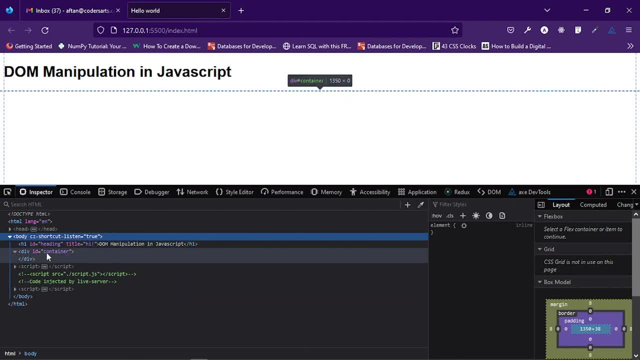 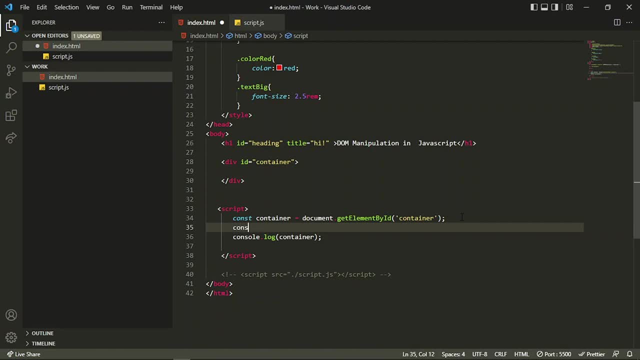 this here, But in this div nothing is there or no element is there. So, basically, how you can create an element, first let's see that. So if you want to create an element, let's say I want to create a paragraph or a p tag, So for that I'll be using documentcreateElement. 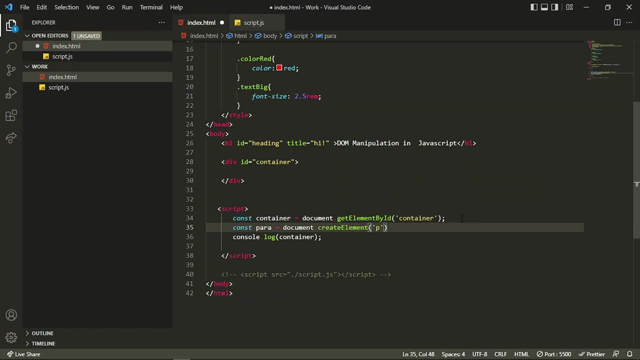 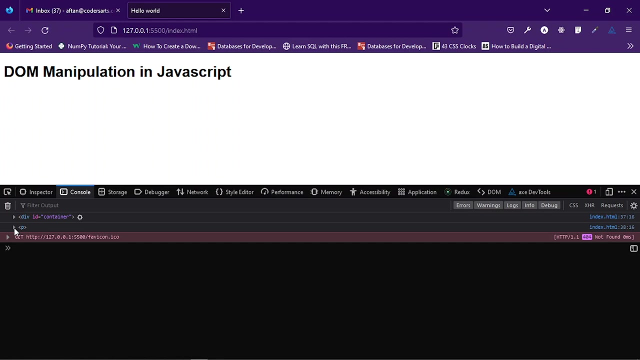 This method will allow you to create any kind of element that you want to create. And now, if I just console log this one, This paragraph here, I think it should be after the container. Let's see what happens. now You can see we have this p tag, But there, 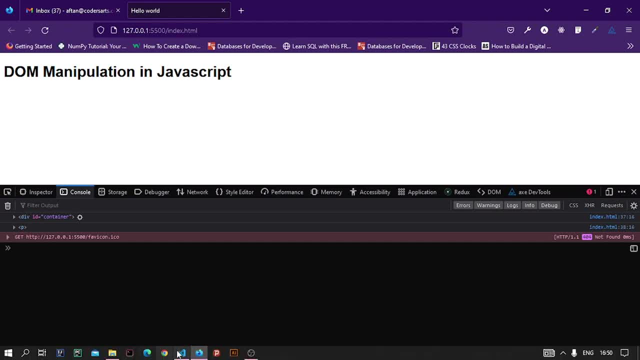 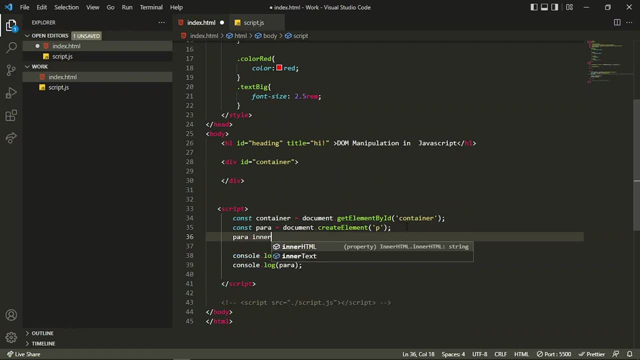 is no content inside this p tag. There is no content inside that. How can we add content inside that? So for that I can use innerstml to add some content inside that, Or I can use the method that we have, paracreateTextContent, or let me just 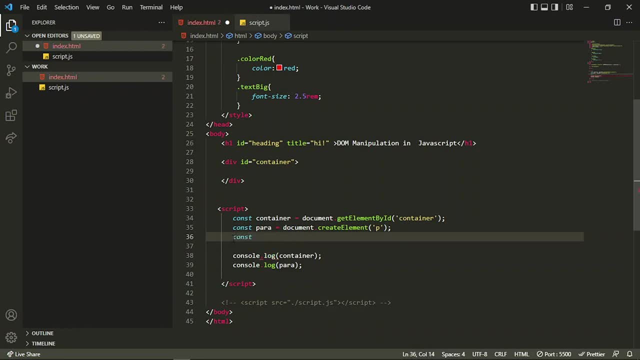 create one text content first, Then I will append that. Let's say, I have this content: DocumentcreateTextContent. So this textNod or this textNod method will allow you to create any content that you want to add inside this paragraph. Let me just create a content here. 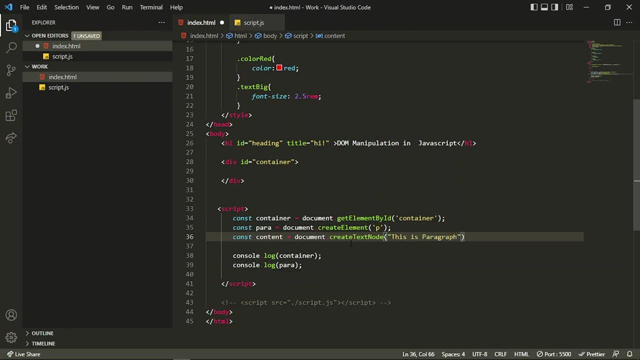 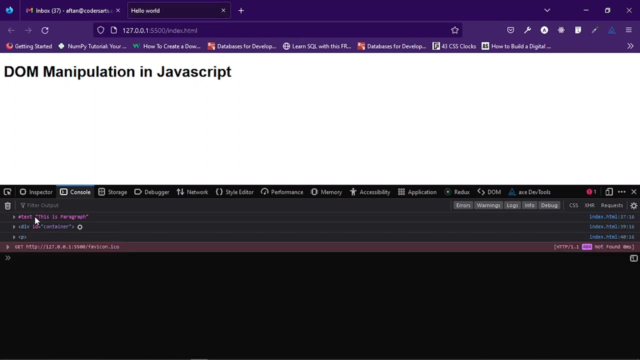 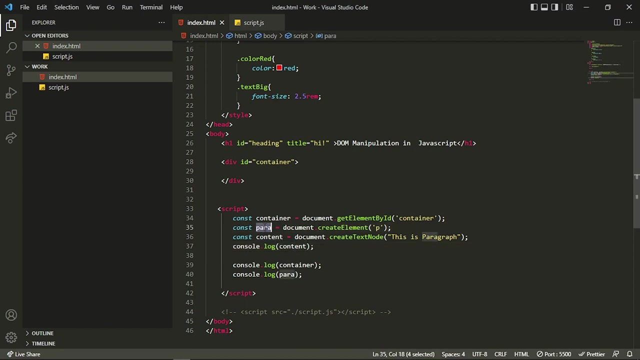 This is a paragraph, So this paragraph. if I console log this, This will be a normal content. If I see that, You can see we have a text content. This is a paragraph. Now, if I want to append this content inside this paragraph tag or this p tag, How can I do that? It is very simple. 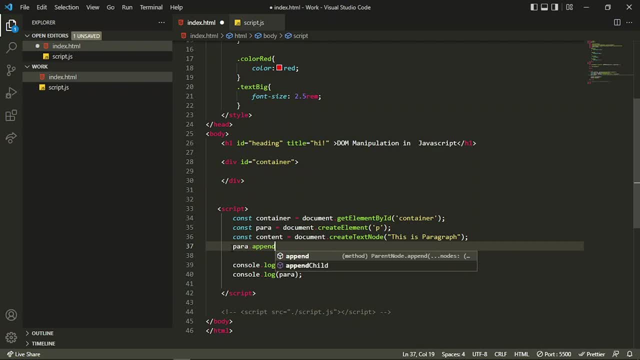 You can just use paraappendChild And you can insert this content that you want to append here. So this appendChild method Allows us to append something inside a element, Or inside an element It can be any text content. It can be any other element that you want to append. That is possible. Now, that is there. 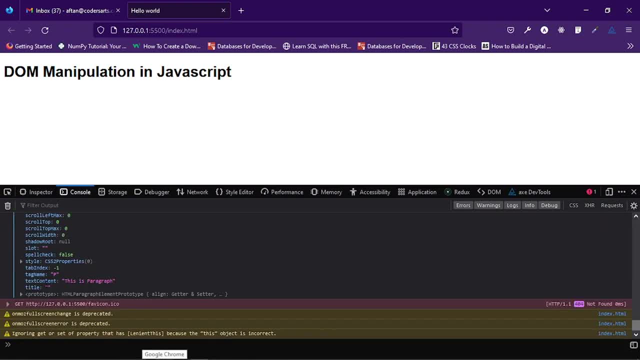 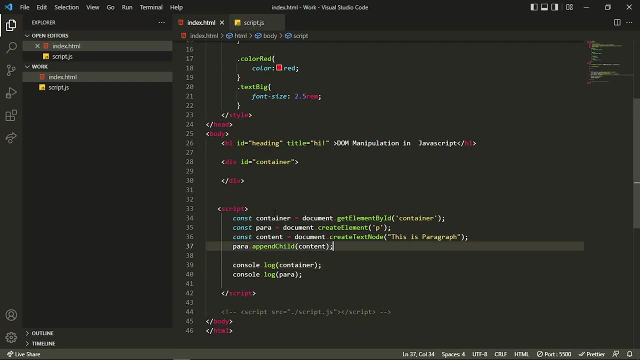 But we are not. We are still not able to see the content. But if we expand this, you can see text content properties there And inside that we have this paragraph method. So it is very easy. You can simply append that And for appending that inside this container, This div, Which 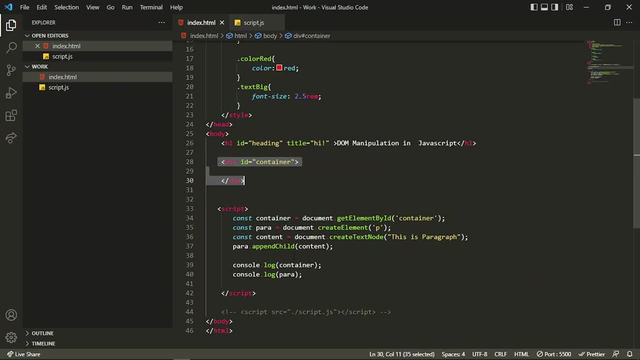 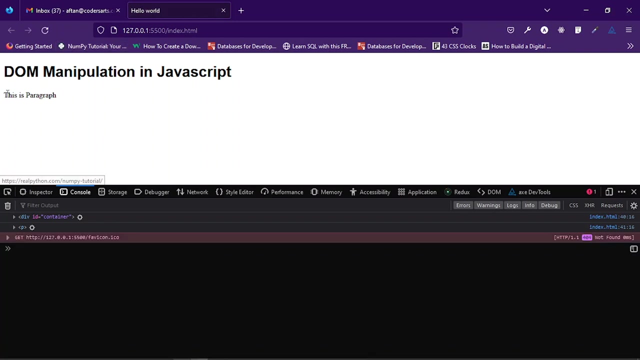 we have here. We will again be using this appendChild, So I can use containerappendChild And inside that I can specify this paragraph. Now, if I see that, It will be visible here. You can see that This is paragraph, If I. 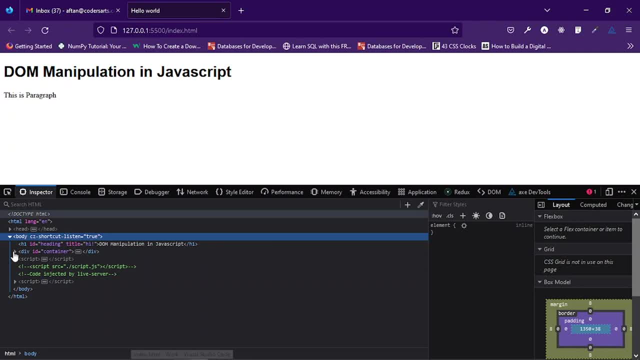 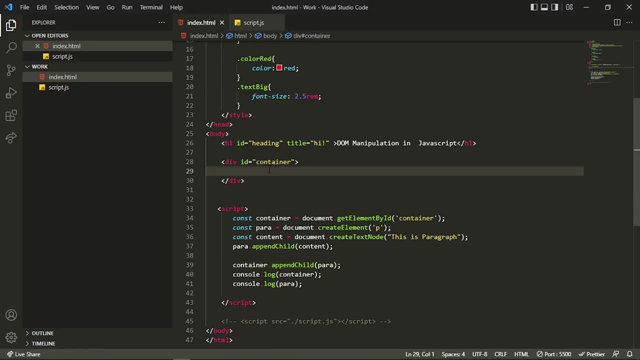 see the inspector. now In The Div Container You can see we have this p tag. This is a paragraph, Let's say. if I have one more div inside here, Let's say it is having an id of para one. 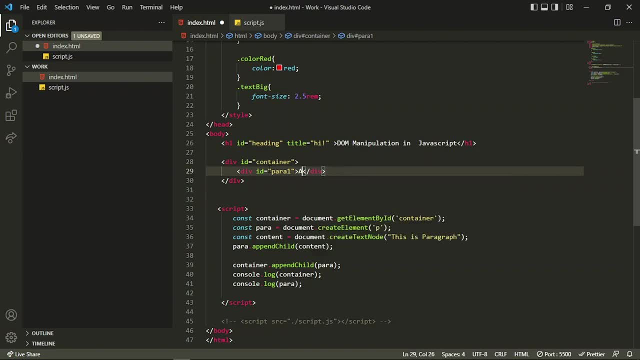 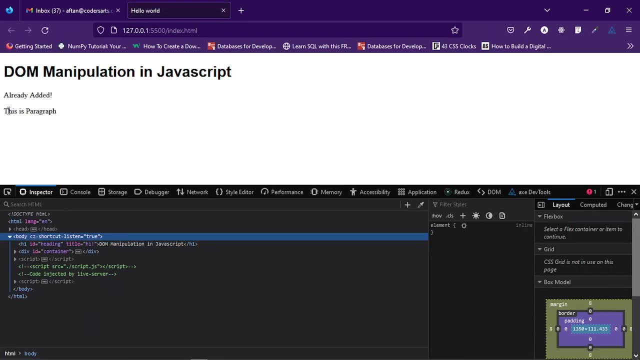 And inside that some- or let's say, already added. Let's say, I have this one, So it will be there, but our newly created or newly appended element is coming at the end. You can see that it is coming at the end. If you want this element to append at the 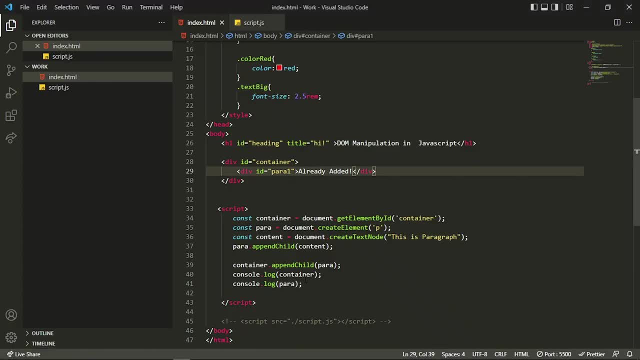 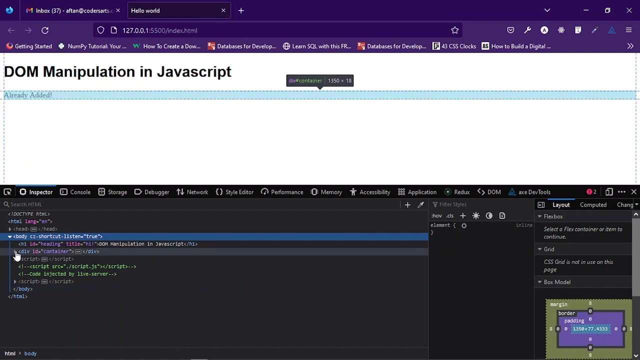 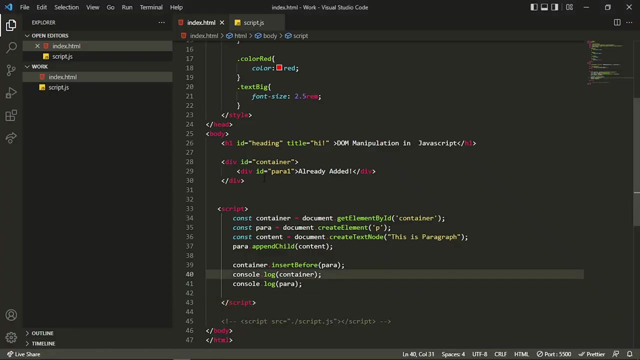 start, not at the end. So you can use insert before. So you can use insert before here. So this will add the element at the start, not at the end. Let's see that. Okay, It's not adding. Okay, I think I need to grab this element first, So then I think that will work. 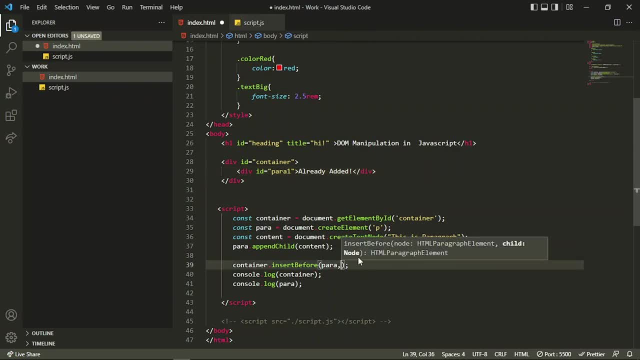 So we have this And we need to specify: Okay, Okay, Okay, So we have this now. So this node is this para comma. let me just grab this element here, para one, and then show you that, let's say, para one, document dot. get element by id. 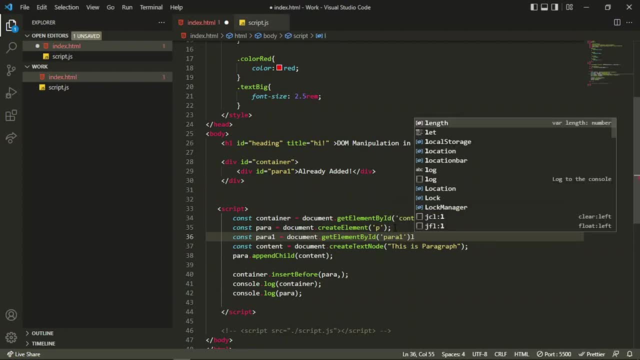 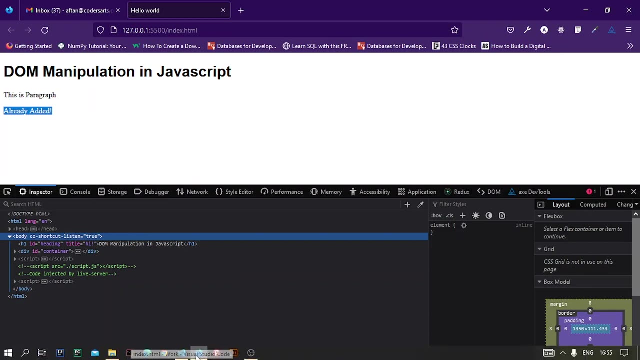 I can specify para one here. So this para one I have to specify as a child. So para one is a child. before that I want this element to be- Now you can see it has added before this element, because earlier I didn't specify the children. 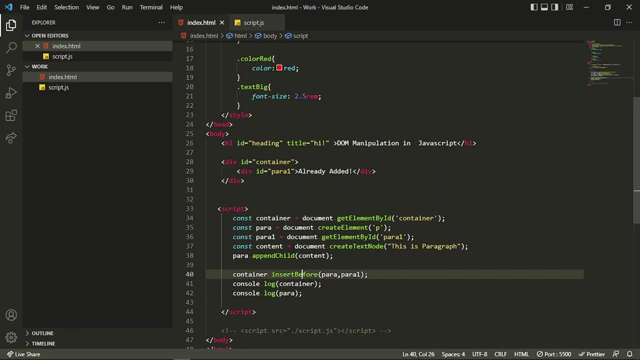 before that I wanted this element to be. that's why, similarly, you can specify other elements and you can specify the element before that you want this element to come, this newly created element to come. So this is one way. similarly, we have other ways to add elements inside the container. 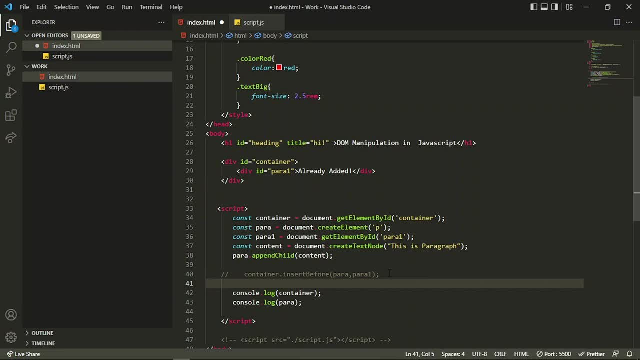 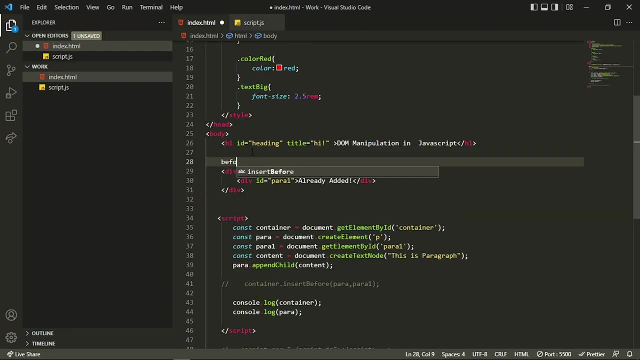 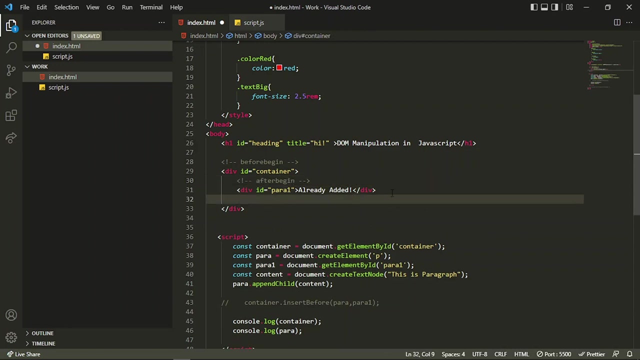 let's add other ways. let's add this paragraph with other ways. we have something called position. this is a position of before begin. we have this position. this is the position of after begin, which means it will be at the start. This is the position before end. 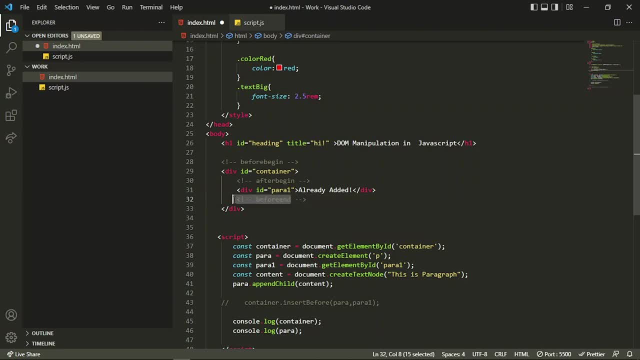 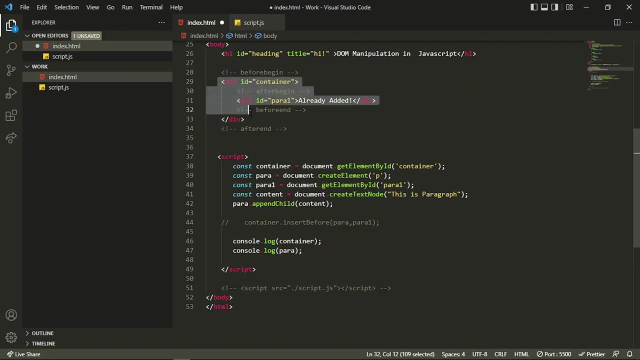 Okay, Comment it out. and this is the position which is after end. So all these four positions are there. where I can specify element to be, I can specify the element before the container. I can specify the element or place the element after- after the children, like after the container started and before all the other children. 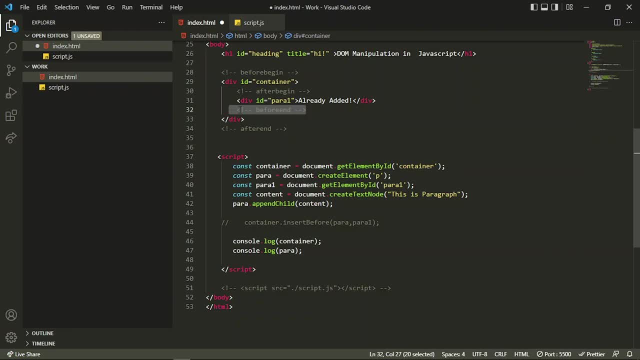 And I can specify it at the last element in the children or in the container after all the children, and I can also specify them at the end or after the end of this container. So after this container is finished, then we can also specify it here. 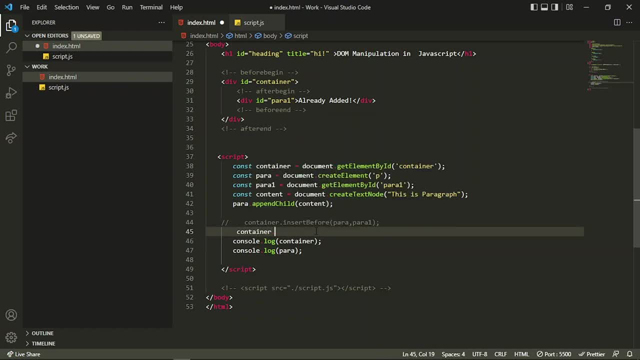 Let's see all the four positions by adding container here. Container is nothing but our this main container div. Now if I use insert Adjacent Element, Then I can specify the position. you can see that where insert position, so I can specify before begin here. 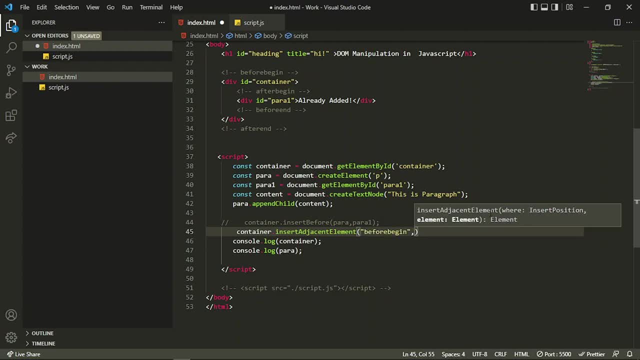 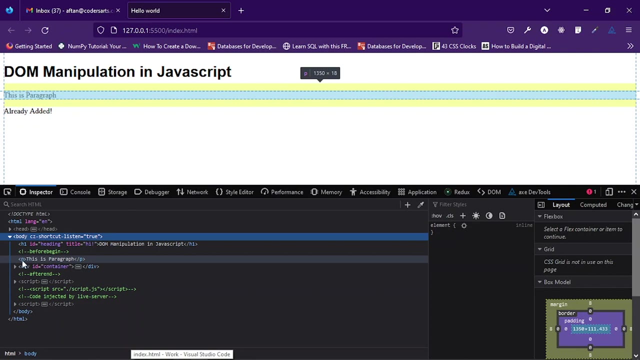 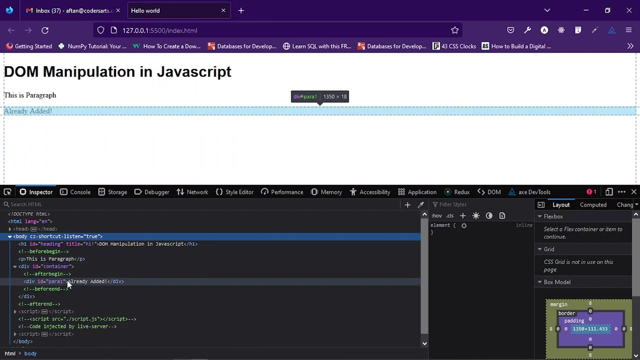 You can see we are suggested here before begin in double quotes and now I can specify the element. so I want the element para to be actually specified. Now you can see in the container, this is the location where this newly created paragraph is added. So it is before this container glass inside that we have this paragraph or the one which 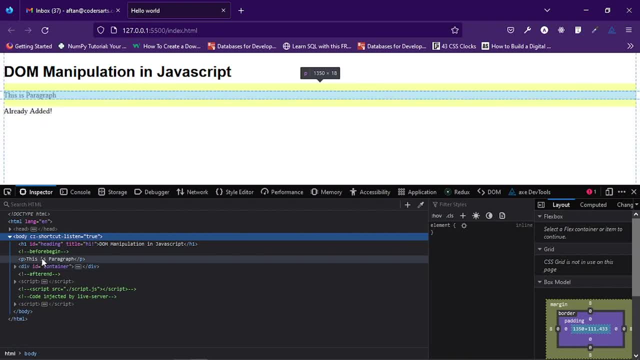 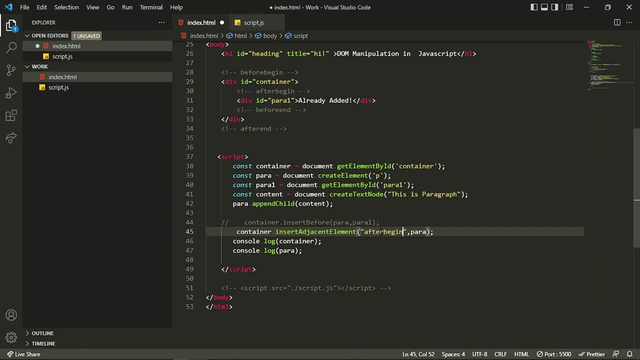 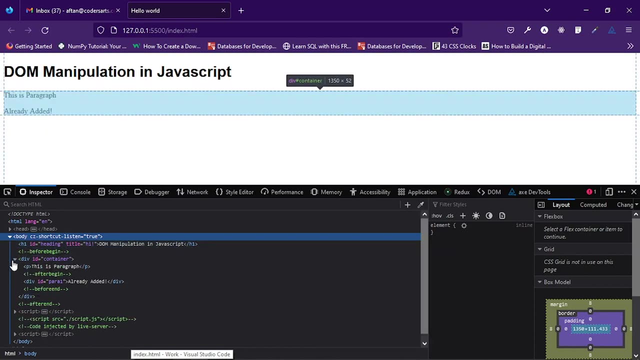 we added by default, and this one is from the JavaScript which is added just now. Similarly, we have this after begin position, so it will be inside the container, but before all the other children. Now, it will be inside the container, but before all the other children. 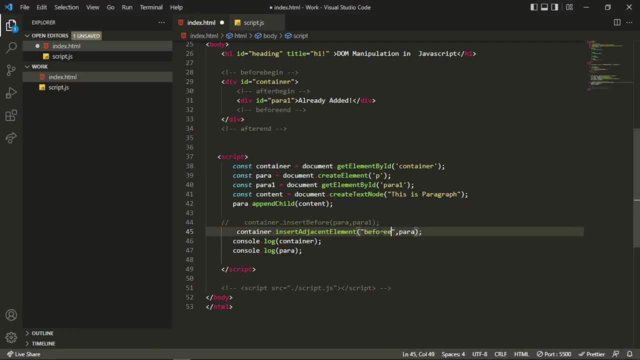 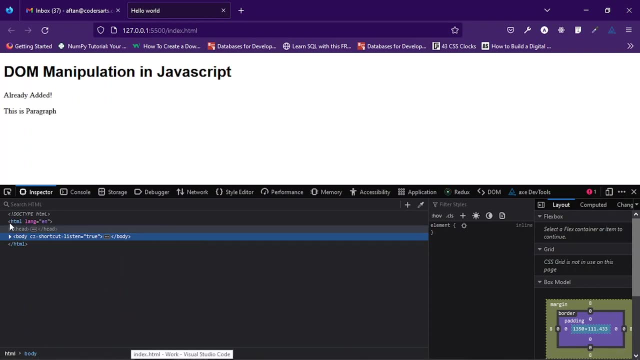 similarly, we have before end, which will be at the last. so it will be at the last in the container. so I think it is not showing me that. let me just expand it. I can see it is at the end, before end. similarly, we have the last position.